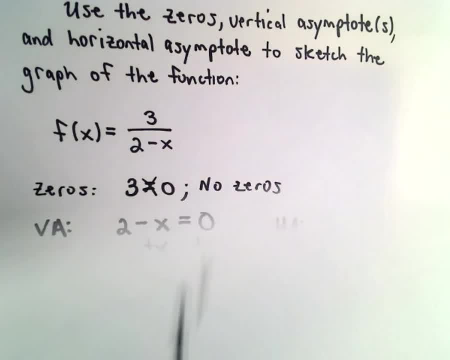 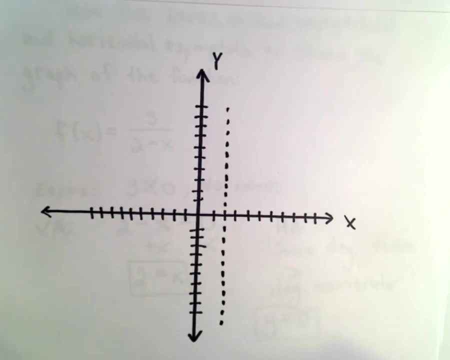 based on that, we don't have a ton of information, I would say, to go on. So let's see: x equals 2 is our vertical asymptote, so let me put that in there. We simply said that there was. 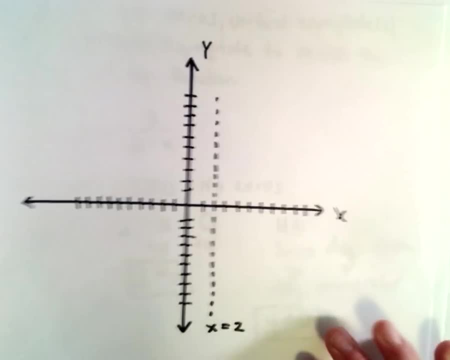 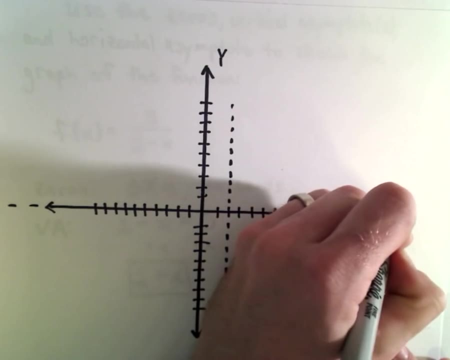 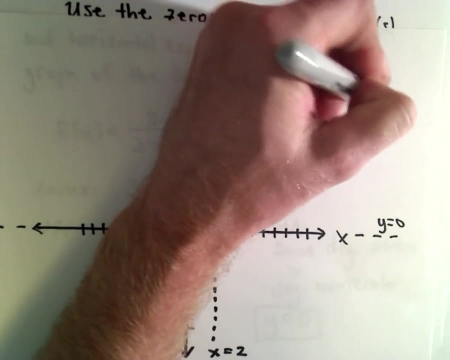 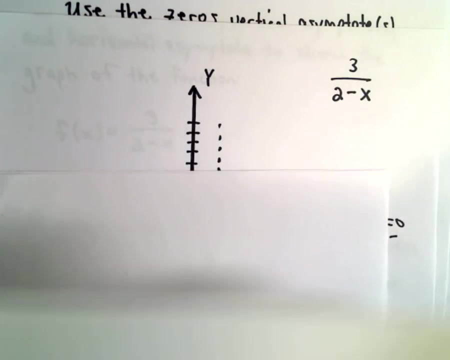 there are no zeros. so we said there's no zeros, Y equals 0, or the x-axis is going to be our horizontal asymptote. But now let's just plot a few points. That's certainly, I don't think is a terrible idea. So let's see, I'm just going to put. 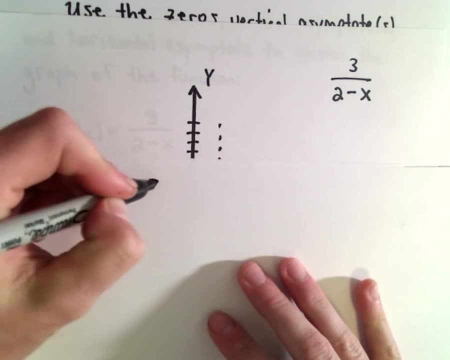 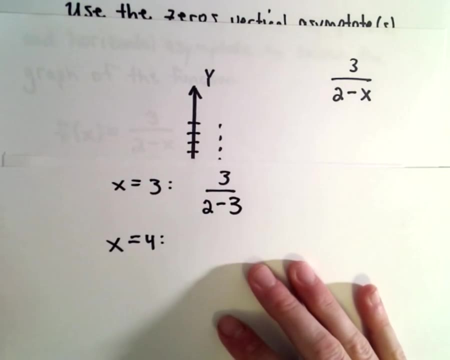 in a couple points. Let's say let's use maybe x equals 3 and x equals 4.. So we would have 3 over 2 minus 3, if I substitute in x equals 3.. Well, that's going to be 3 over negative. 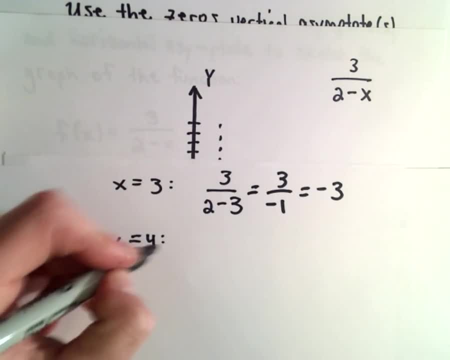 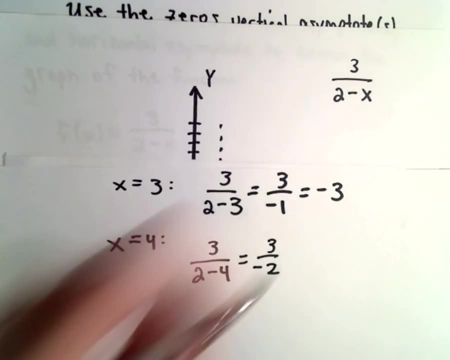 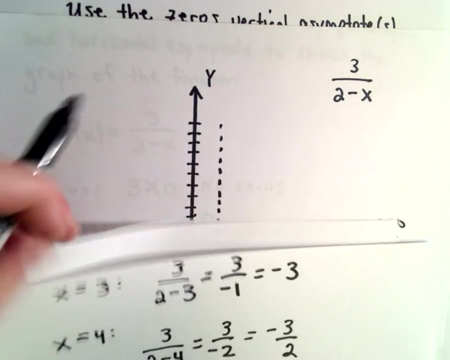 1, or negative 3.. x equals 4,. that'll give us 3 over 2 minus 4,, which will be 3 over negative 2, or negative 3 halves. So let's see here I'm going to put those values in there. So at negative 3, excuse. 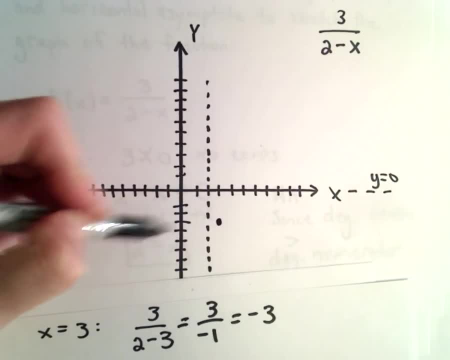 me, at positive 3, we get negative 3.. And at x equals 4, we're at negative 3 halves. So let's see that's 1 and a half. So somewhere right there And you can keep. 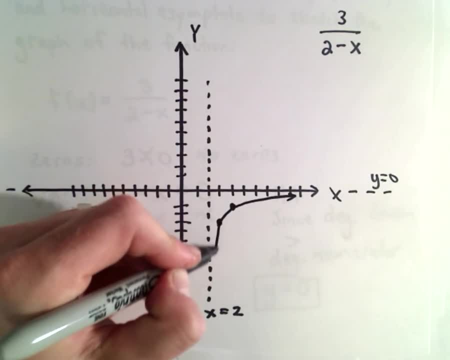 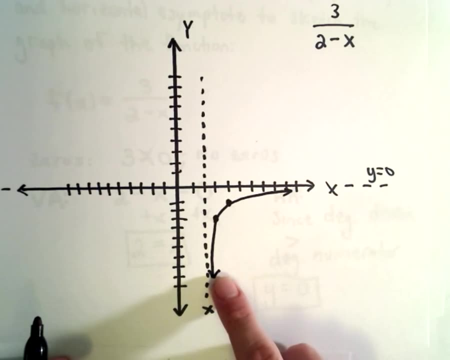 Plotting points And you'll see that your graph the bottom right portion of it. again, it gets close to that horizontal asymptote and it gets close to the vertical asymptote. I know it doesn't cross the x-axis again, because we know that there's no 0's. So again, 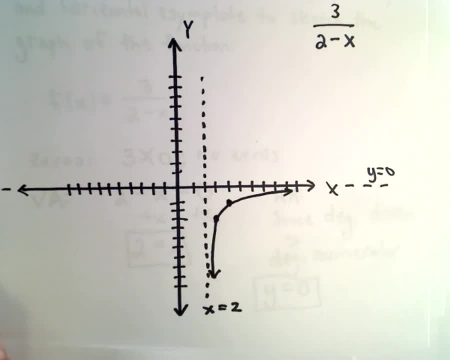 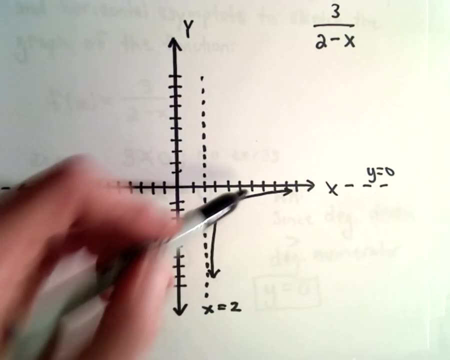 remember, a rational function can cross its horizontal asymptote. It doesn't have to, like this example shows. It can cross a horizontal asymptote, But again, in this case we said no zeros, which means it doesn't cross. So let's see. 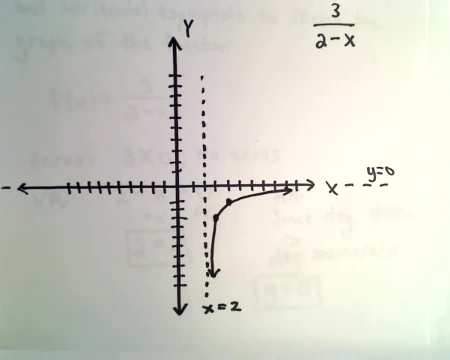 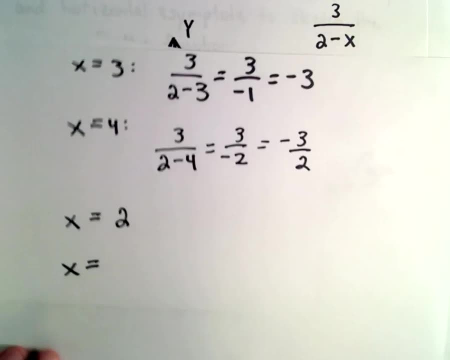 We could also let's plot maybe two more points. Let's use 2 and 1.. I think you'll see we've got a little bit of symmetry here, At least about- excuse me, not 2, because that'll give us. we know that that's undefined, So let's use x equals 1.